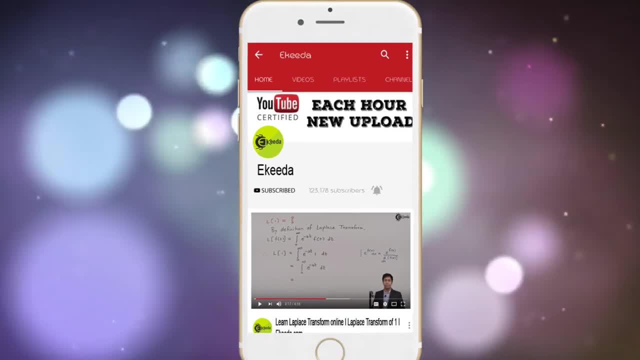 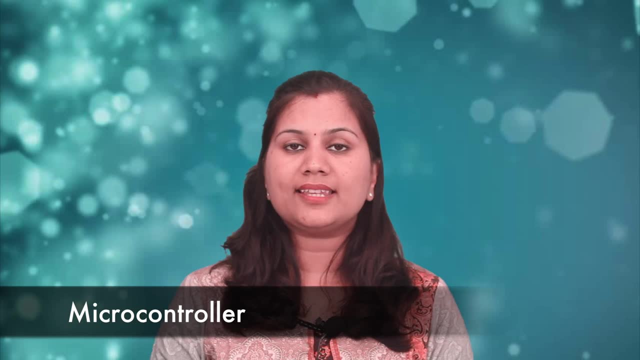 Do subscribe to eKIDA channel and press bell icon to get updates about latest engineering, HSE and IIT-JEE main and advanced videos. Hello friends, in this video we will study that- what is a microcontroller? So let us start with the topic. 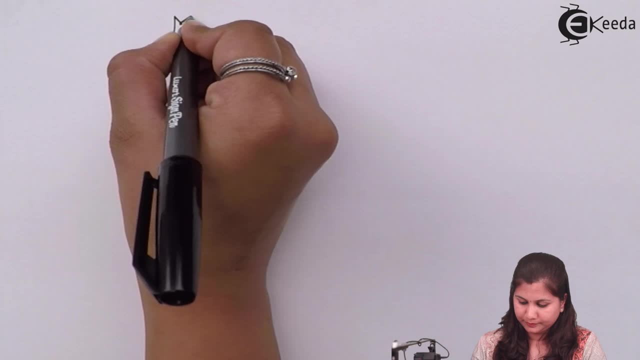 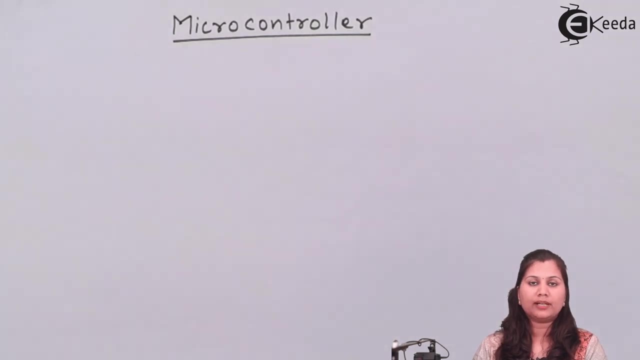 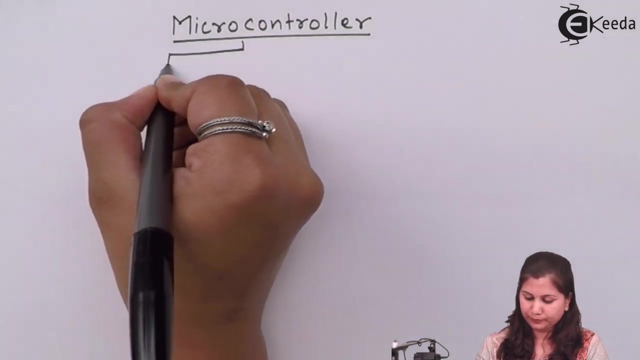 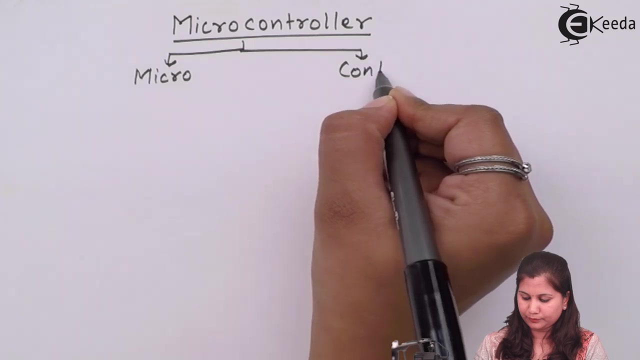 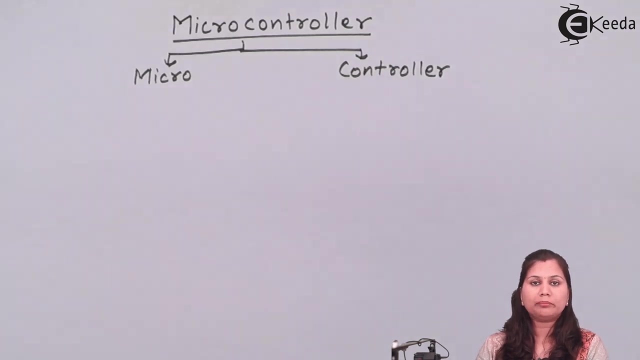 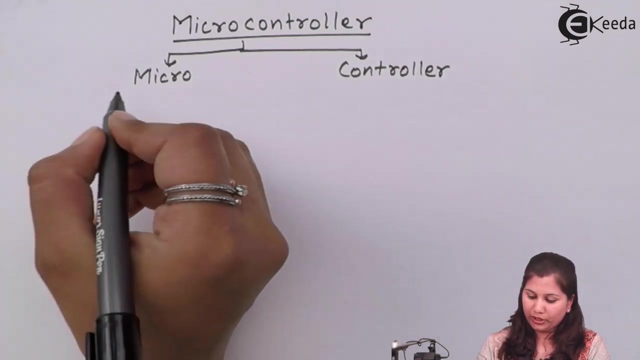 This word microcontroller. it is composed of two terms: micro plus controller. Micro means very small in size, Micro means very small in size And controller means a device which controls the operations of all the devices. So here we have the word micro for small. 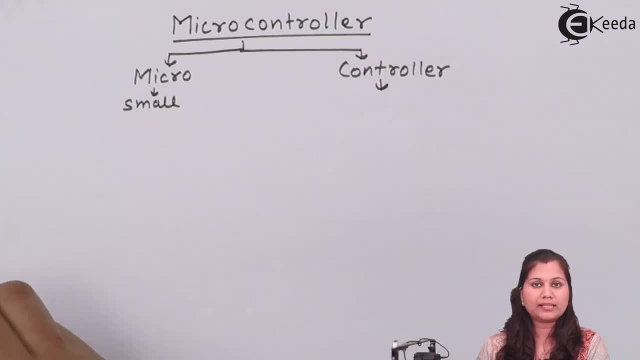 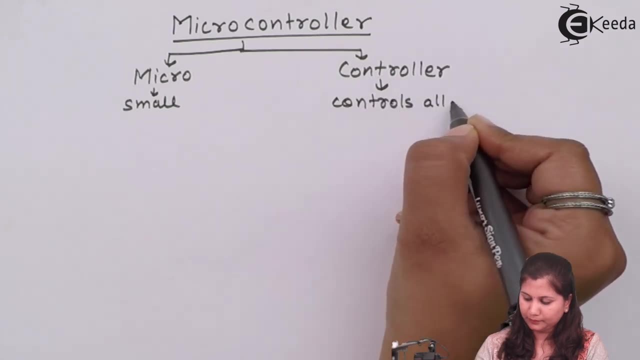 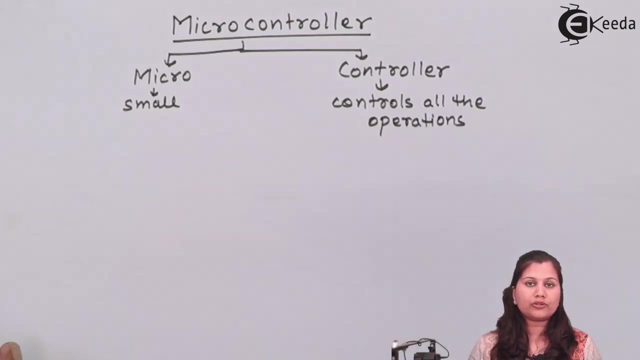 And controller means controls all the operations. So microcontroller, we can say that they are the devices which are very small in size and they control the operations of all the other devices. Now, microcontroller, a general microcontroller. it consists of various components. 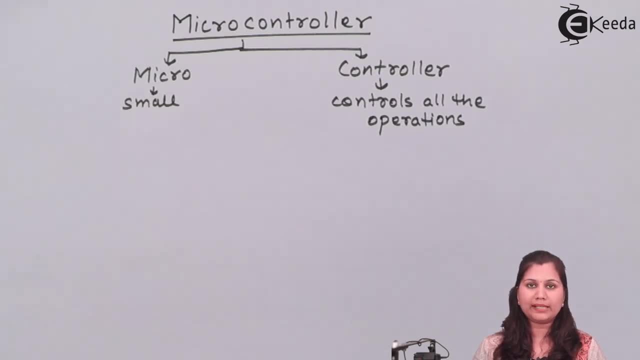 It consists of various components, Like memory is there and this memory can be either RAM or ROM. RAM is the random access memory and ROM is the read only memory. So this microcontroller, it can have memory, It can have serial input output ports. 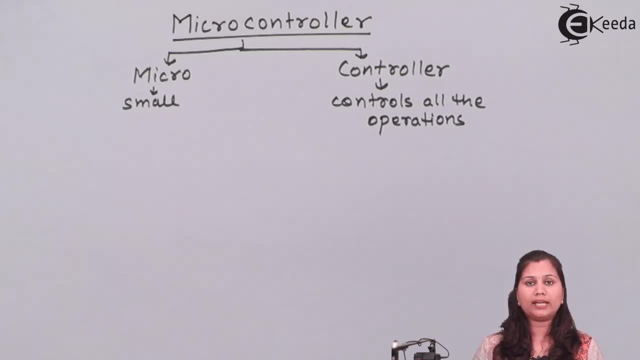 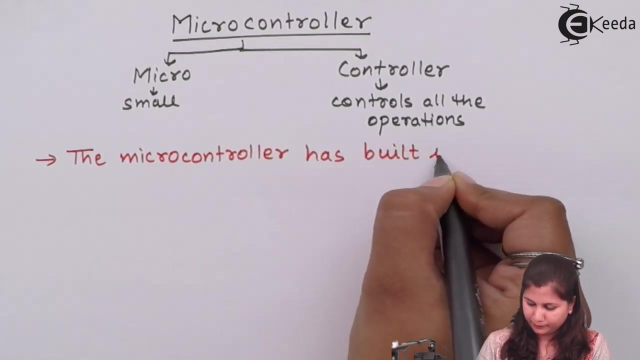 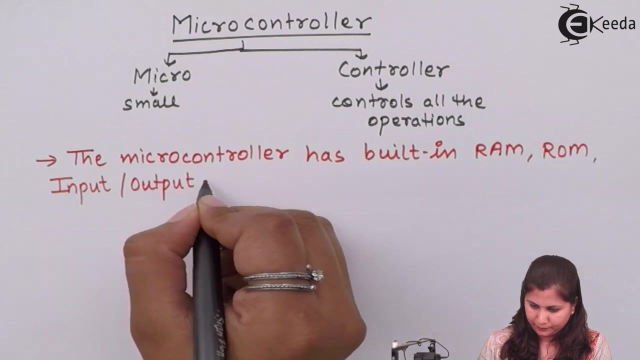 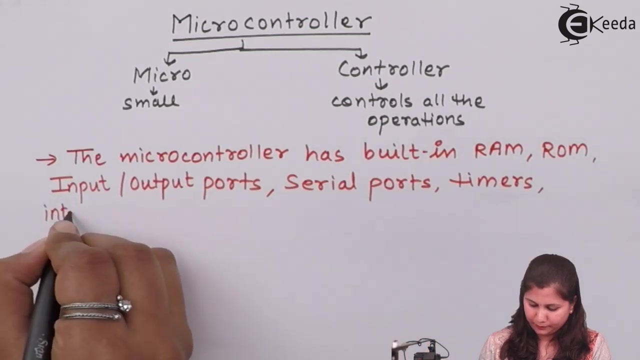 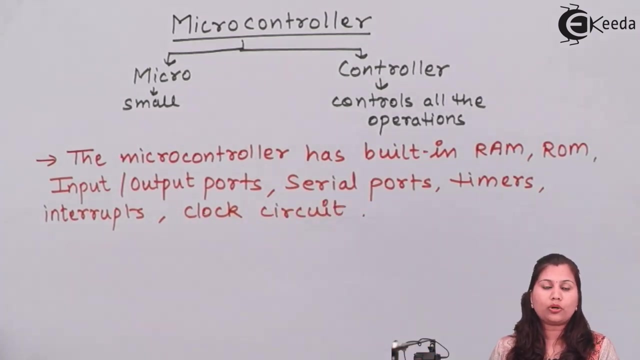 Also it can have the peripheral devices and timers and counters. All those are there in the microcontroller. So we can say that a microcontroller, it generally consists of all these components. So a microcontroller, talking about its components, it will have built-in RAM, ROM, input, output ports, serial ports, timers, interrupts and clock circuits. 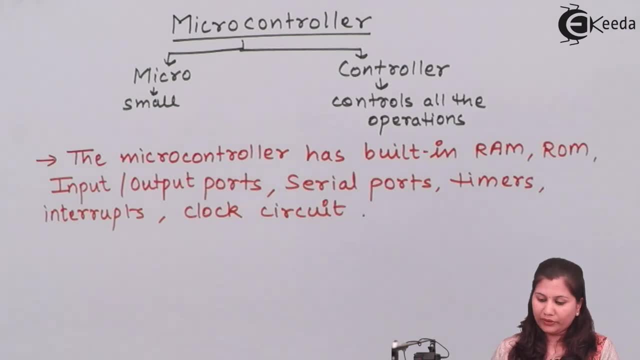 All will be present in the microcontroller. So we can say that microcontroller it is nothing, but it's an on-chip computer. Okay, All the devices of the computer, they are embedded on a system. They are embedded on a single chip. 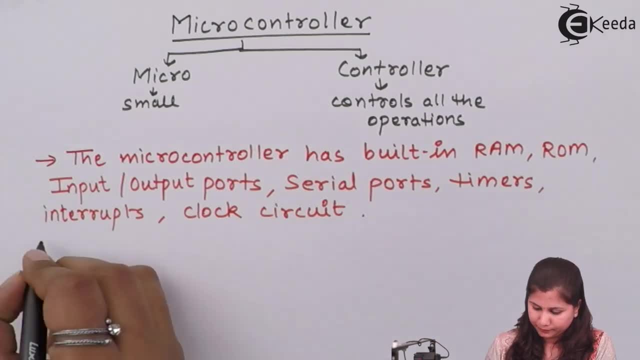 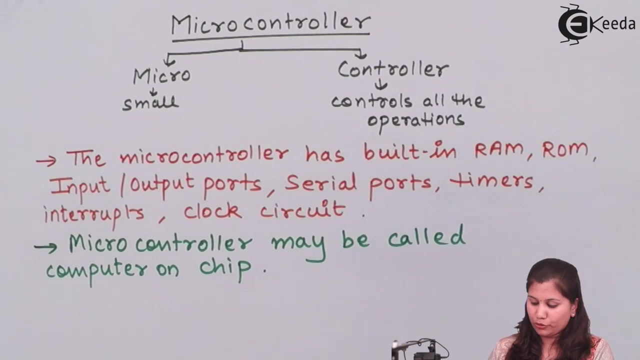 That will be called a microcontroller. So another name for microcontroller is the on-chip computer, Because it is having all the components which are embedded on a single chip. Now, if we compare this microcontroller with the on-chip computer, So we can compare this microcontroller with the microprocessors. 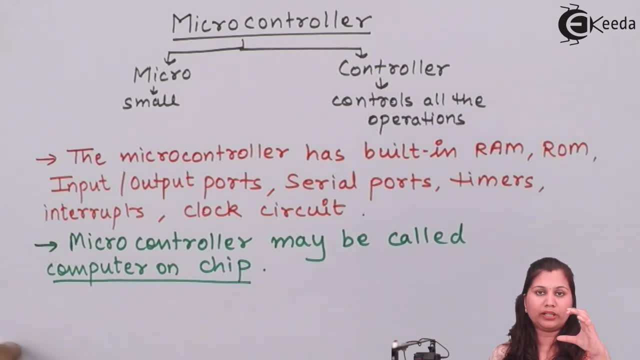 So microprocessors, they are having the central processing unit, that is CPU. They will have a separate memory, separate block for the input output ports and separate block for the interrupts, timers and clock circuits. So everything is separate on that microprocessors. 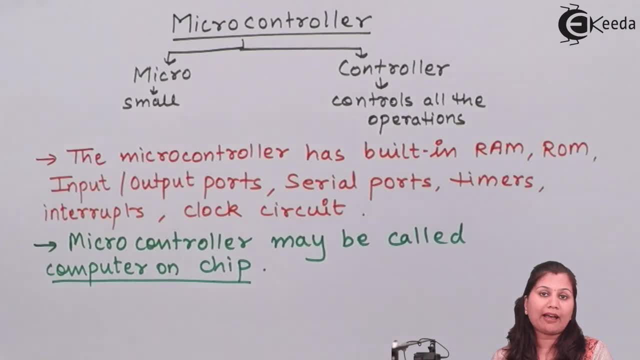 But in the case of microcontrollers because it is having all the things on one chip. So we can say that all the features of the microprocessors they are contained in the microcontroller. So microcontroller it is comprising the features or it has the microprocessor plus. it has the memory section and the input output section also. 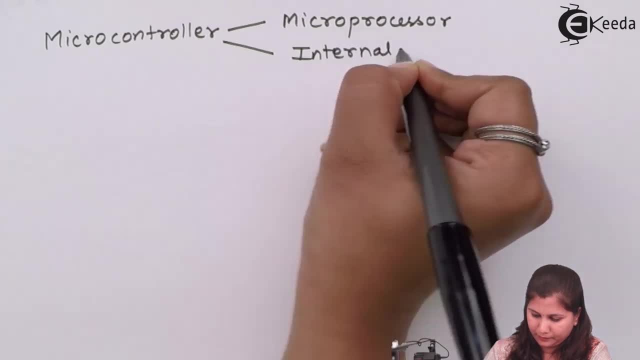 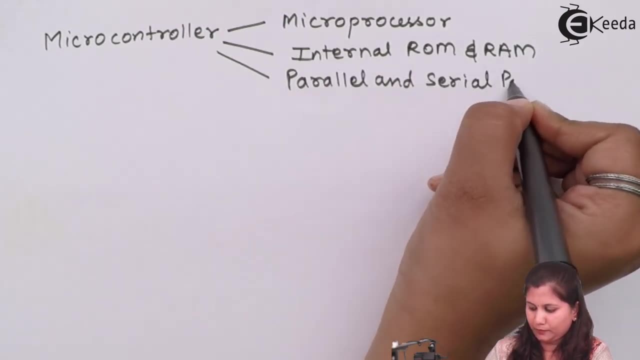 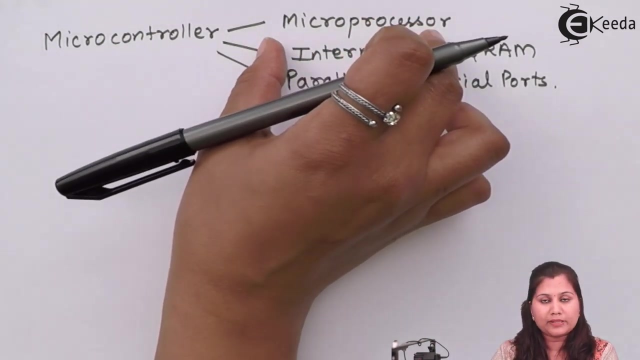 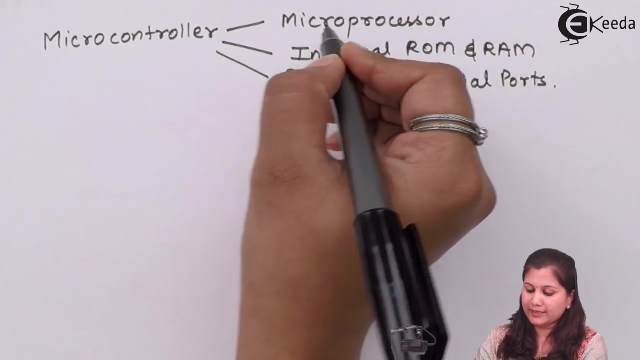 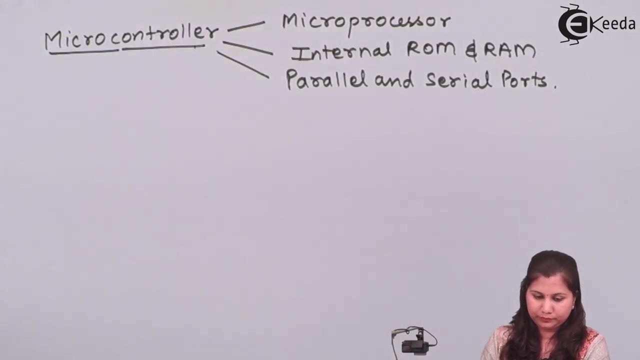 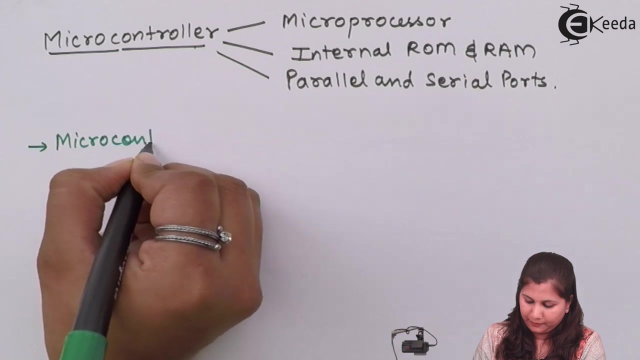 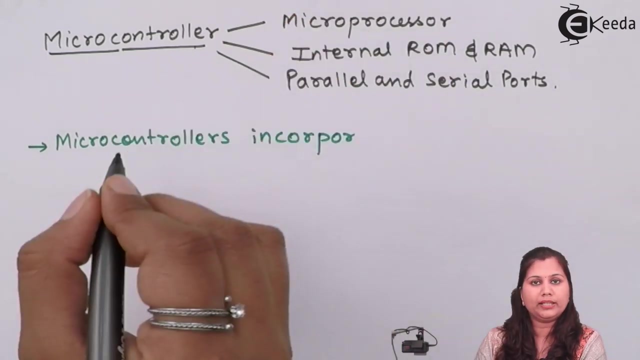 So all the components of the microcontroller. they are in the microprocessor, plus the internal ROM and RAM and the parallel and serial ports. So if we combine all these things we will find out the microcontroller. So we can say that microcontrollers incorporates all features of the microprocessor. 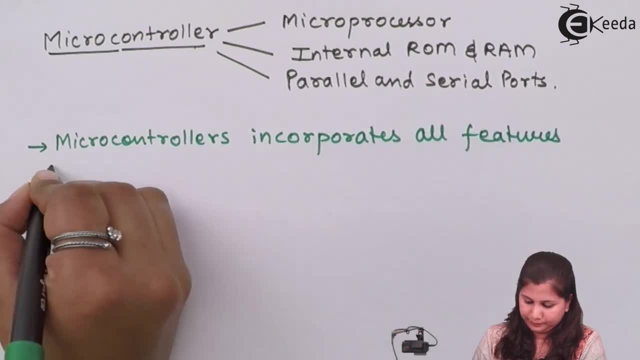 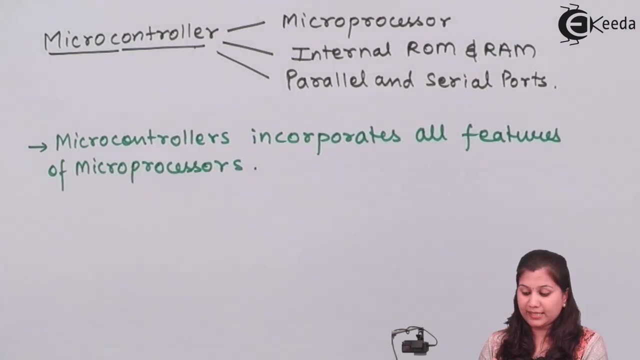 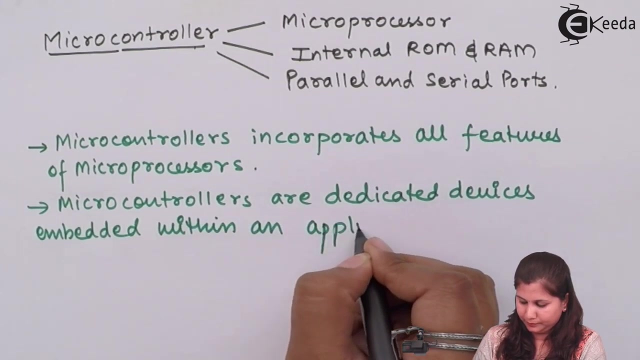 Now as the microcontroller, because it is a type of controller, It is controlling the microprocessor. So we can say that microcontrollers they are having all the things on one chip, They are controlling all the functions, So they are very powerful devices. 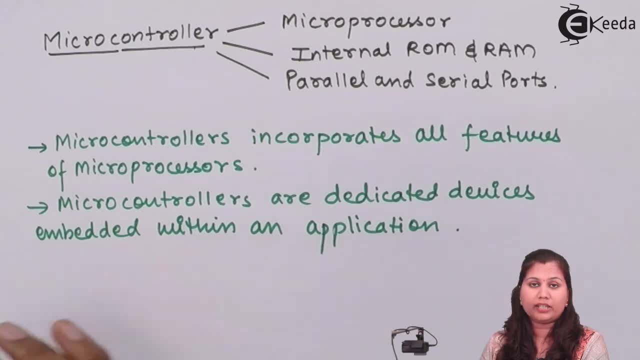 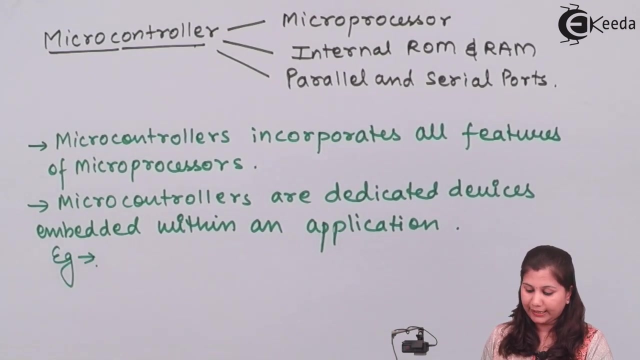 So as they are controlling the functions, so when the microcontrollers, they are used in any application, So they will act as the dedicated devices which are controlling all the functions. If we take an example here, the example of this is like a microcontroller. 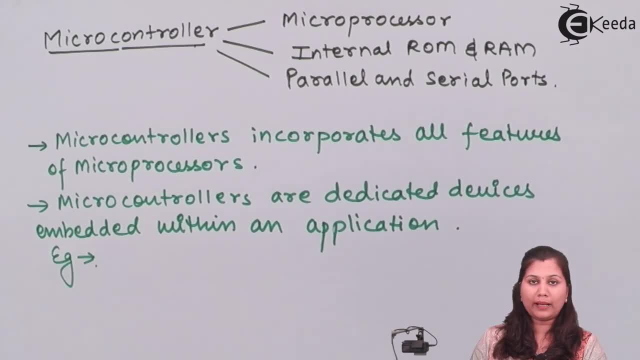 They can be used as the engine controllers in the automobiles. They are also used in the washing machine, in the VCD players and in the microwave ovens for controlling the temperature there in the ovens. If we want to control the temperature, that is done by the microcontroller. 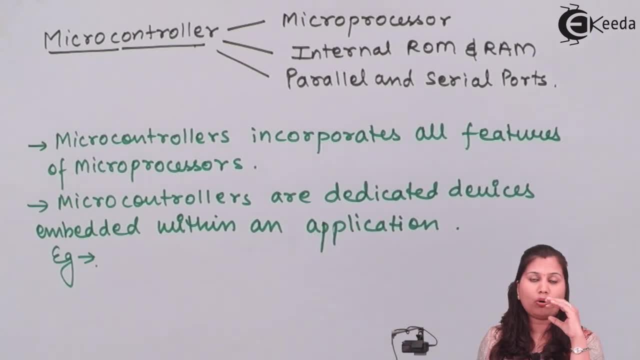 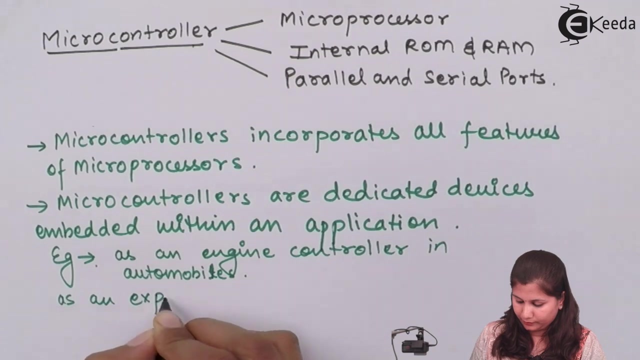 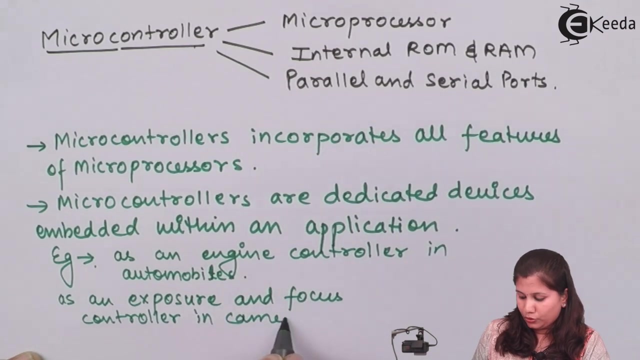 So for any specific task. if we want to use some device for a specific task, we use the microcontrollers. So as an engine controller in automobiles, Also as the exposure and focus controllers in the cameras also, the microcontrollers are used. So in all the applications where controlling is required, microcontrollers can be used. 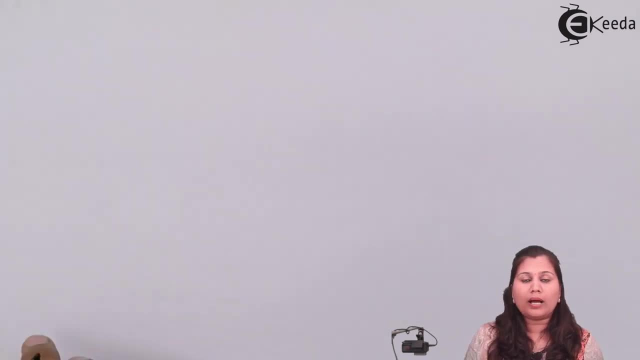 Now as the microcontrollers. it has all the devices Which are embedded on the single chip, That is, the memory and the input output ports, serial ports, timers, counters, all are present on a single chip, So for their manufacturing the CMOS technology is used. 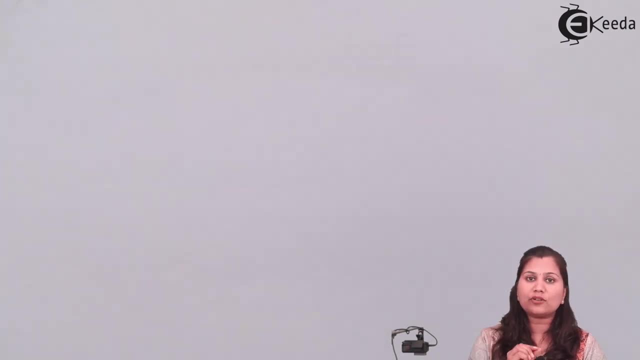 And due to the CMOS technology, the size of these microcontroller is very small. That is why the word micro is there, That is, microcontrollers. they are very small in size Because we are using the CMOS technology And all these small devices. they are embedded on the same chip. 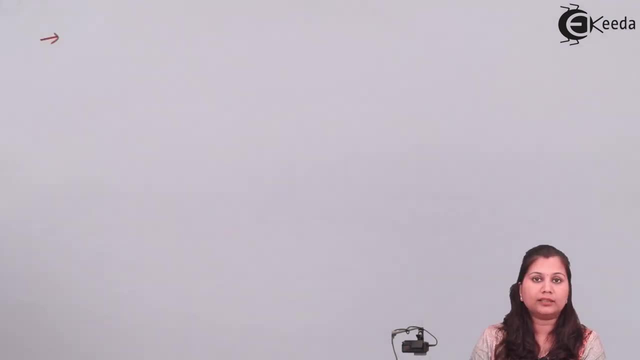 So these on chip peripherals, the input output ports, serial ports. They are selected according to the task performed by the microcontroller in a particular application. So if we want to use the microcontroller for automobiles, We will have the different operations have to be performed. 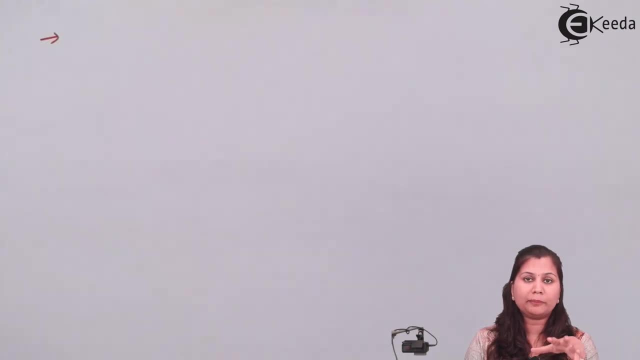 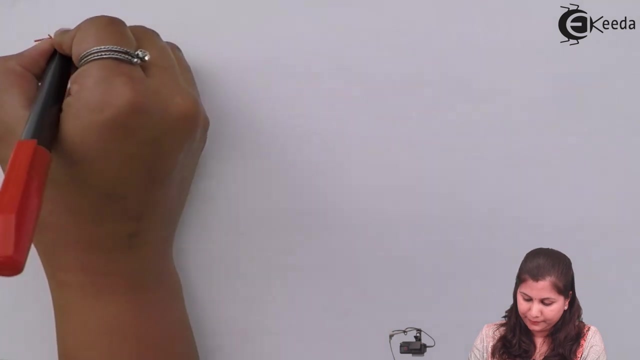 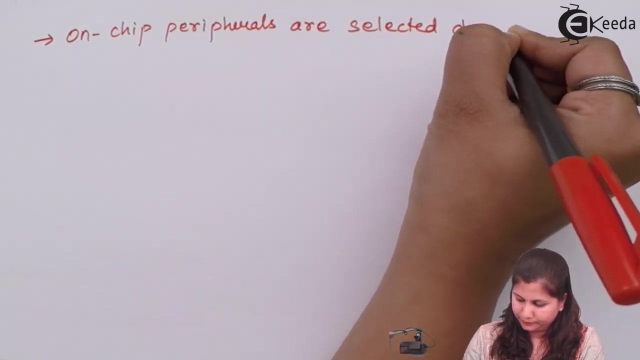 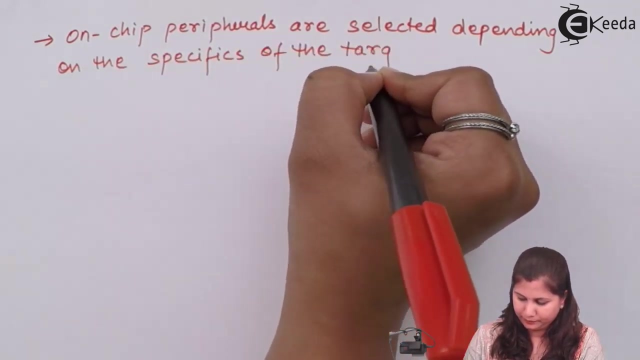 For microwave ovens, different operations are to be performed, So for depending upon the applications, the peripherals are chosen. So we can say that on chip peripherals they are selected according to the task performed in the application. So that is why we are using this chip. 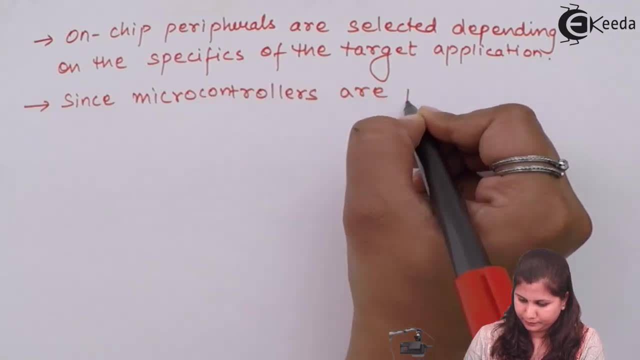 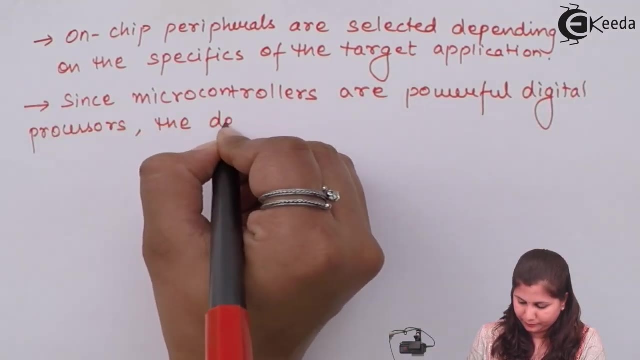 And we can do the same thing for a product. So let's see what what we are doing here. The first we are doing is to take a separate chip. We will put it in the chip and let it work, And you will see this way how the chip will work. 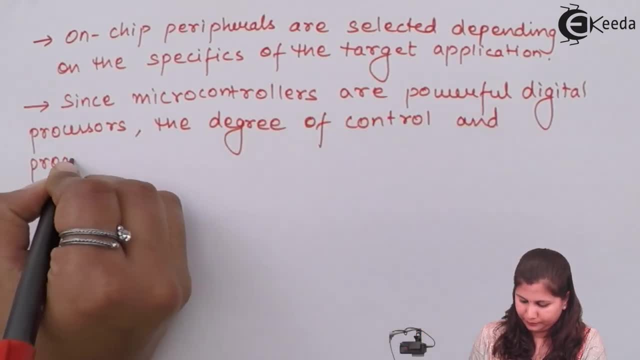 So let's say, this is a chip that is now connected to the PC and we have to put it in the chip. And now this one is connected to the PC. And then we put it in the chip, And now it is connected to the computer. 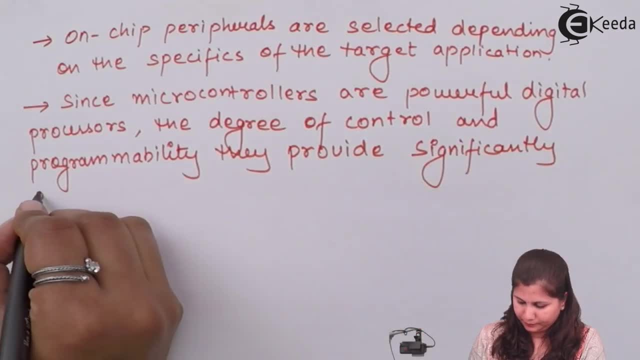 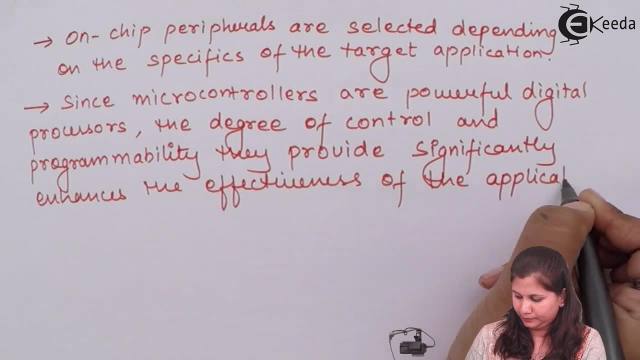 And here you can see it is connected to the PC. If you can see that these are connected to the computer, And now you can see it is dzień down here. So on-chip peripherals, they are selected depending upon the specifics, that is, specifications. 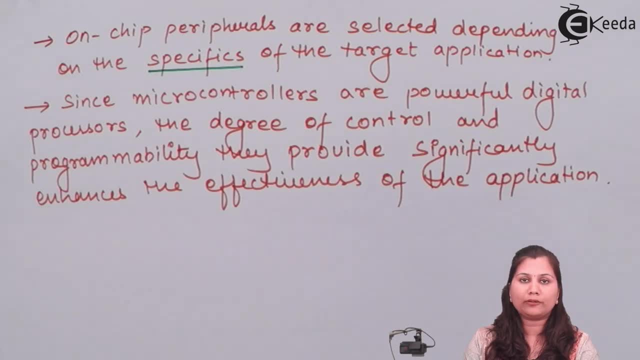 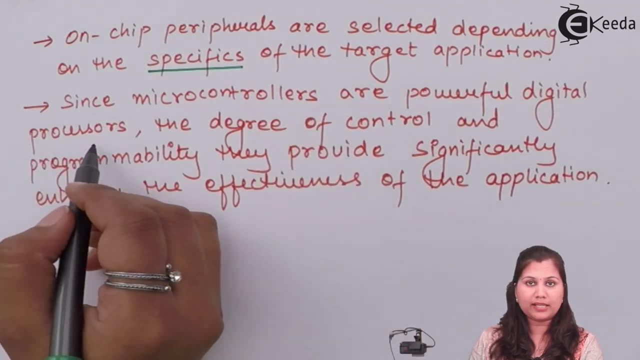 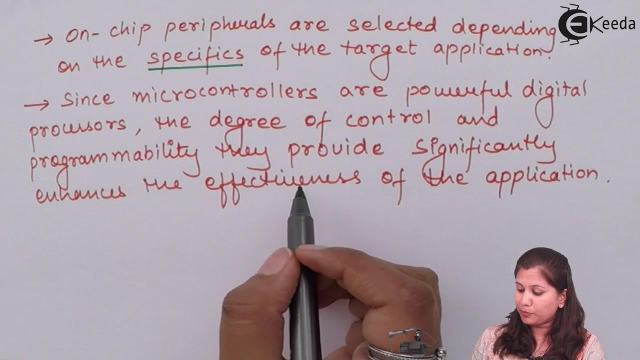 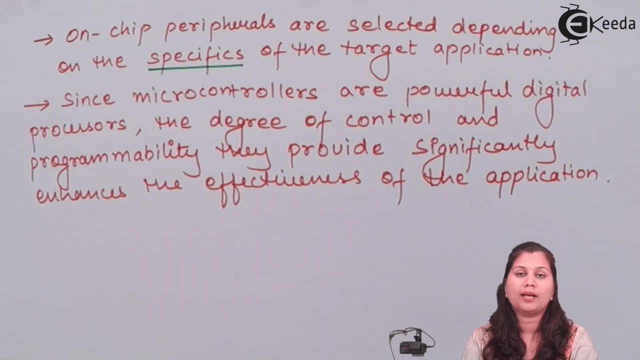 of the target application, for which application the microcontroller is to be used. Now, as these microcontrollers- they are powerful devices, digital processors, so the degree of control provided by these microcontrollers and the programmability it is going to significantly enhance the effectiveness of the application. 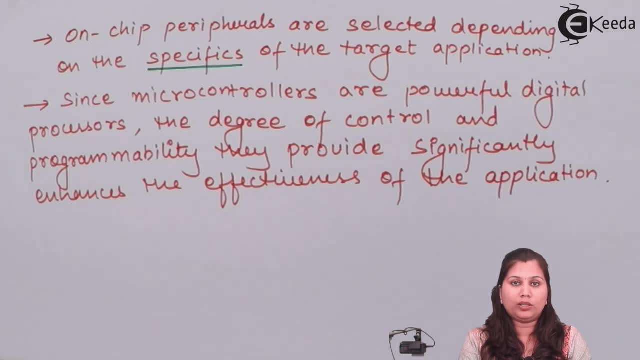 Because if, in an application, if we are using a microcontroller in place of a microprocessor, the effectiveness or the efficiency of the application will be increased. in the case of microcontroller, Because they are very powerful devices, digital processors, so they are going to significantly. 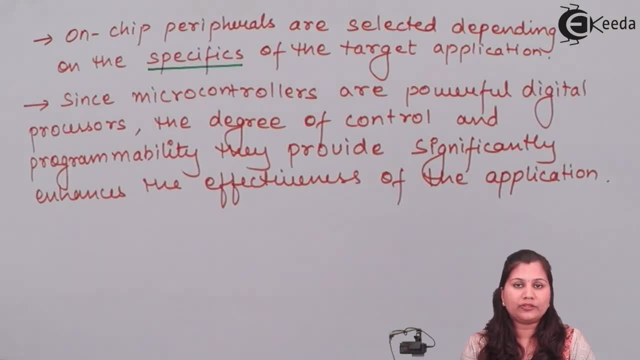 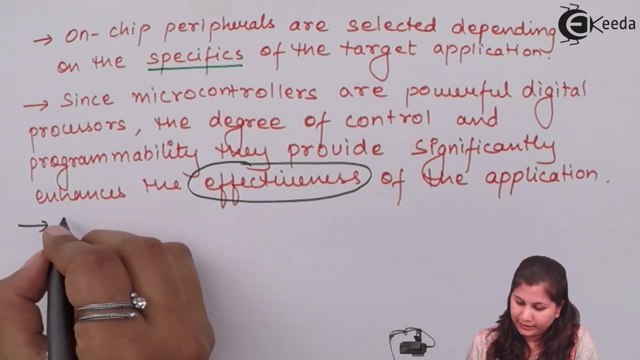 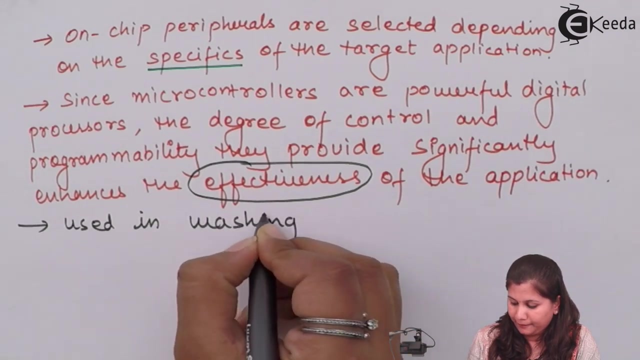 help the same process and they can better control the operations of the applications. So these microcontrollers, we can say that they increase the efficiency of the application. Now, different applications of this microcontroller. We know that they can be used in washing machines. 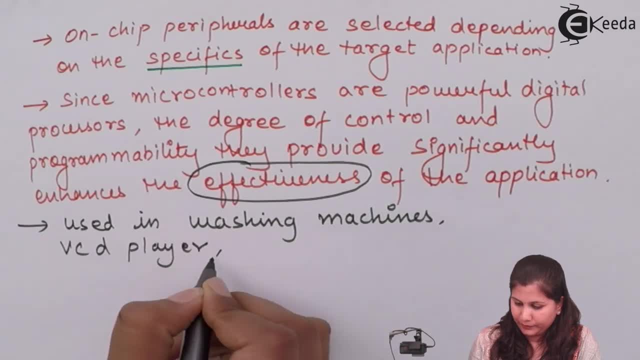 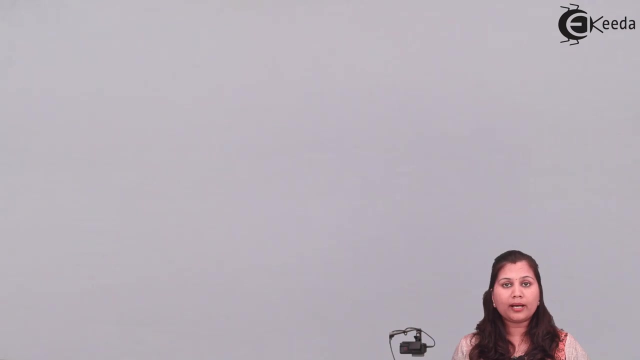 Hey, in microwave oven, in robotics also, microcontrollers are used, and in industries also microcontrollers are used. so these are the various applications of the microcontroller. we have the applications in the robotic field also and in the industrial field also. okay, now talking about the development of the microcontrollers, the intel company it. 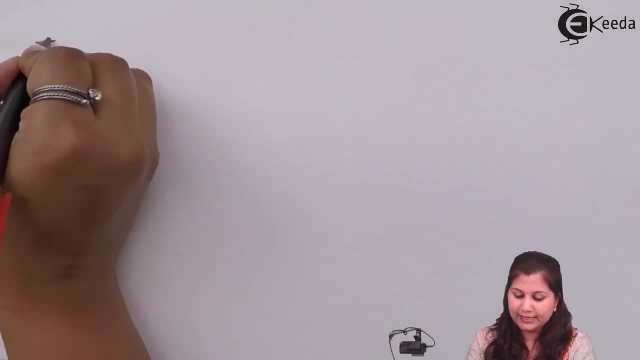 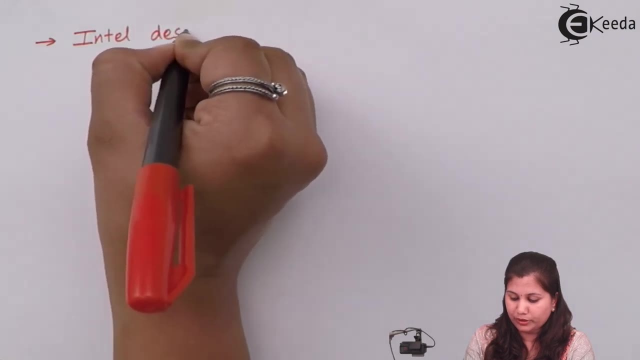 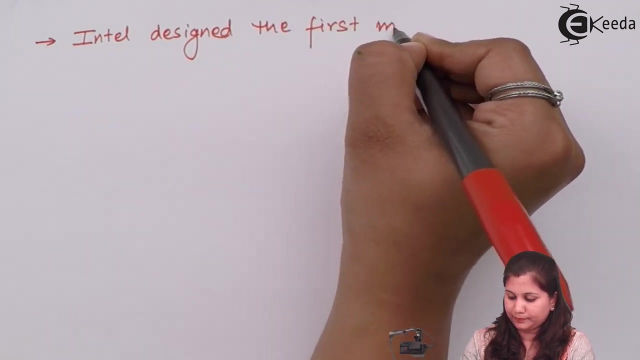 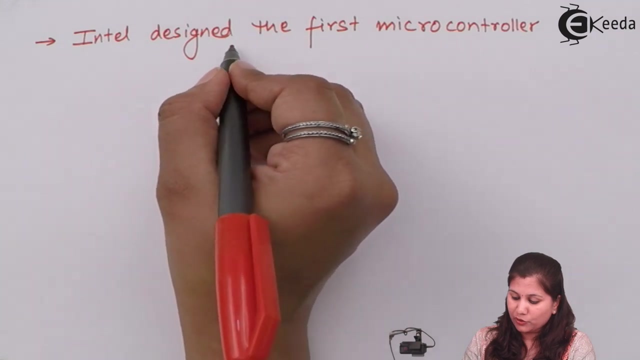 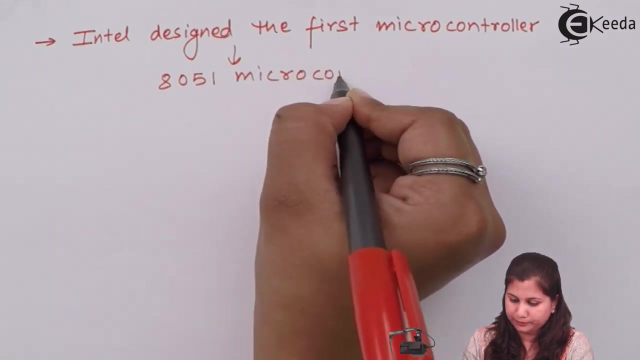 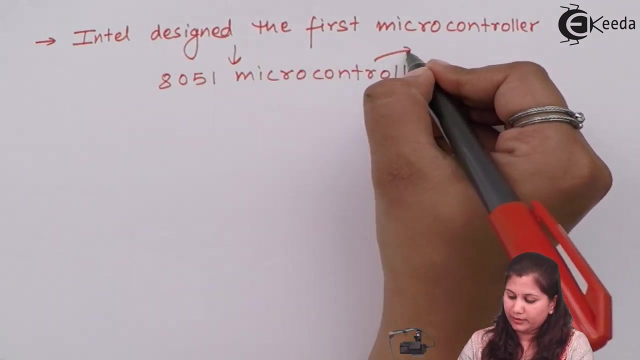 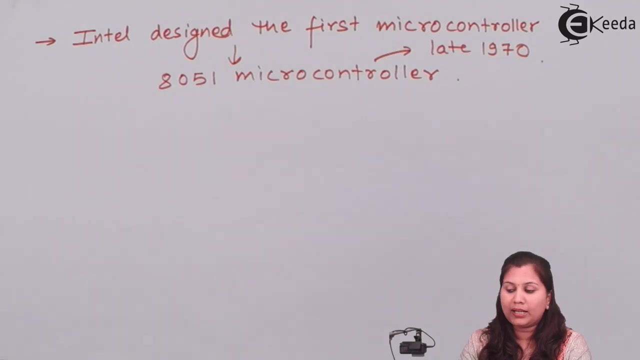 designed the first microcontroller, which is the 8051 microcontroller. intel designed the first microcontroller and this first microcontroller is known as 8051 microcontroller. this microcontroller was developed in late 1970s, means in 1980s, we can say 1981. it was developed by the intel. 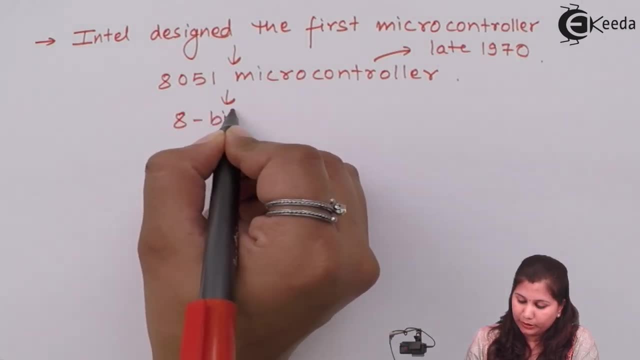 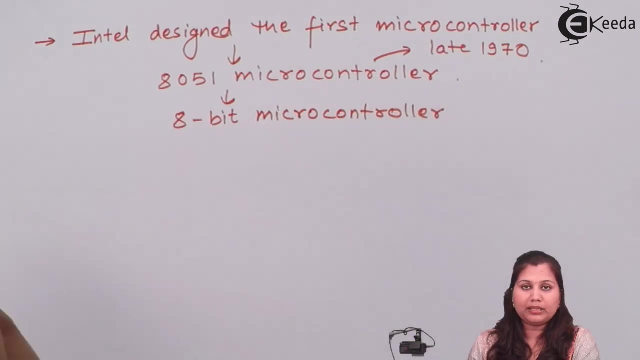 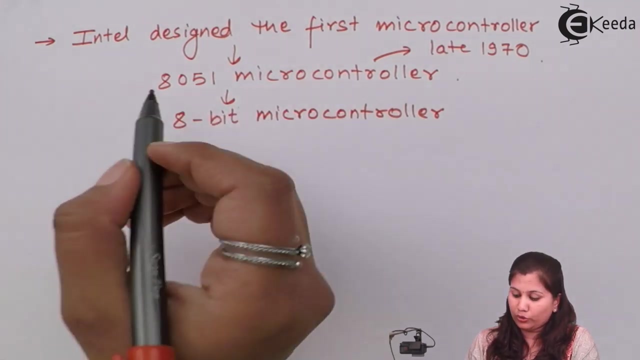 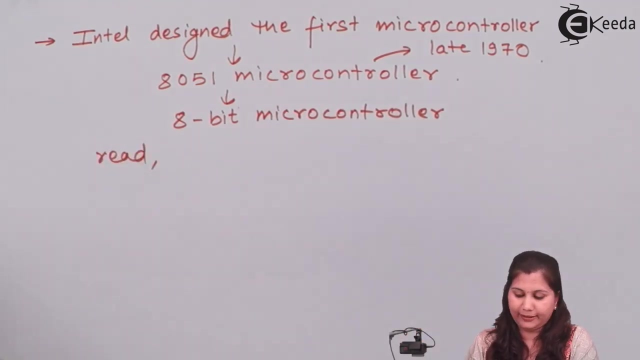 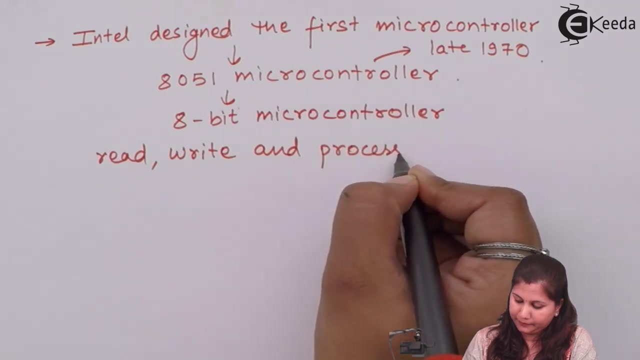 and this microcontroller. it is an 8-bit microcontroller. 8-bit microcontroller means we can classify these microcontroller on the basis of the bits processed by them. so 8051 is an 8-bit microcontroller, means it can read, write and process 8-bit data.